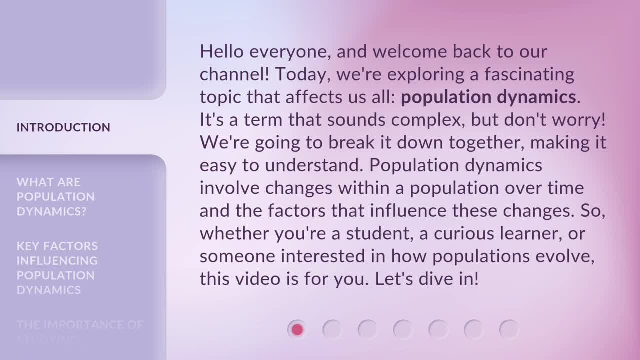 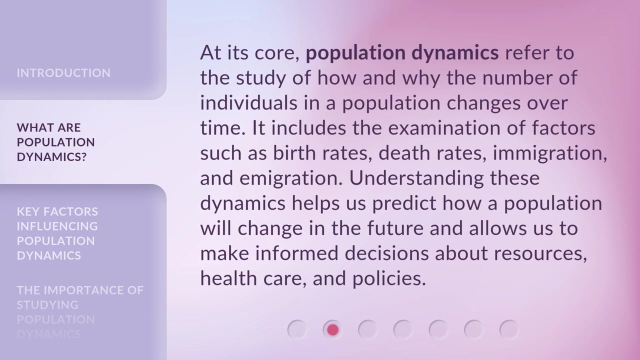 Population dynamics involve changes within a population over time and the factors that influence these changes. So, whether you're a student, a curious learner or someone interested in how populations evolve, this video is for you. Let's dive in At its core. population dynamics refer to the study of how and why the number of individuals 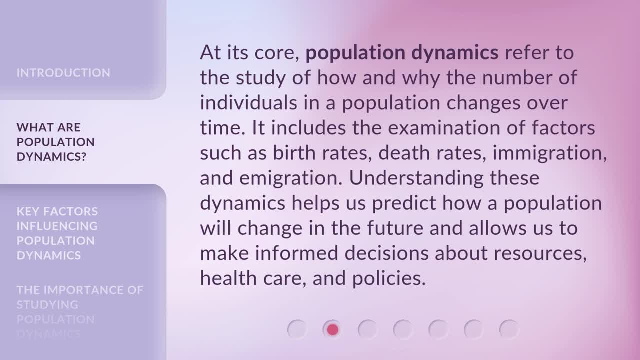 in a population changes over time. It includes the examination of factors such as birth rates, death rates, immigration and emigration. Understanding these dynamics helps us predict how a population will change in the future and allows us to make informed decisions about resources, health care and. 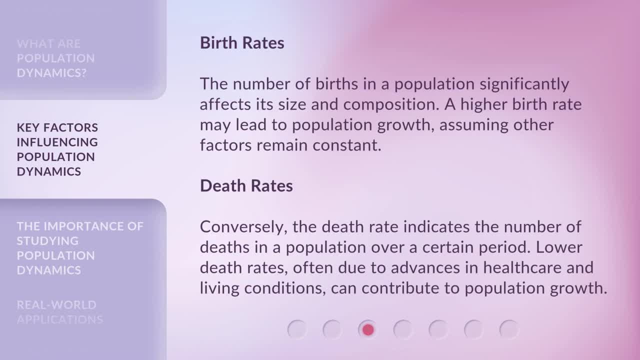 policies. Birth rates – The number of births in a population significantly affects its size and composition. Birth rates – The number of births in a population significantly affects its size and composition. A higher birth rate is a factor for the population's growth. A higher birth rate is a factor for the population's growth. 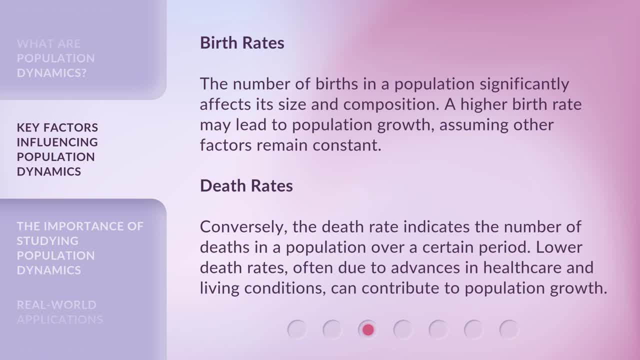 birth rate may lead to population growth, assuming other factors remain constant. Death Rates Conversely. the death rate indicates the number of deaths in a population over a certain period. Lower death rates, often due to advances in health care and living conditions, can contribute. 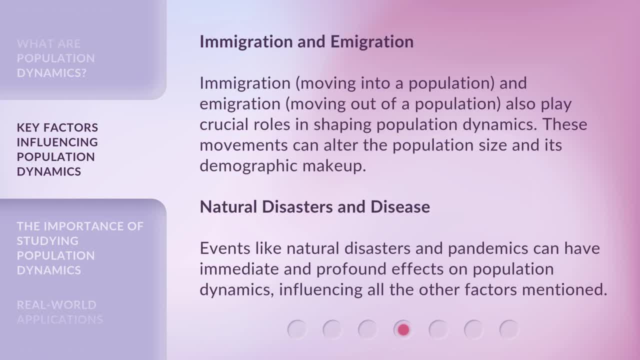 to population growth, Immigration and emigration. Immigration- moving into a population and emigration moving out of a population also play crucial roles in shaping population dynamics. These movements can alter the population size and its demographic makeup. Natural disasters and disease. Events like natural disasters and pandemics. 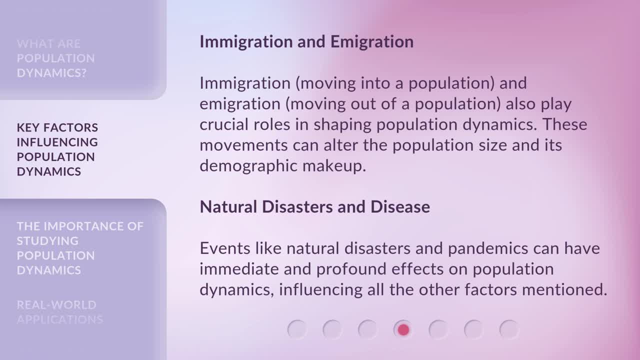 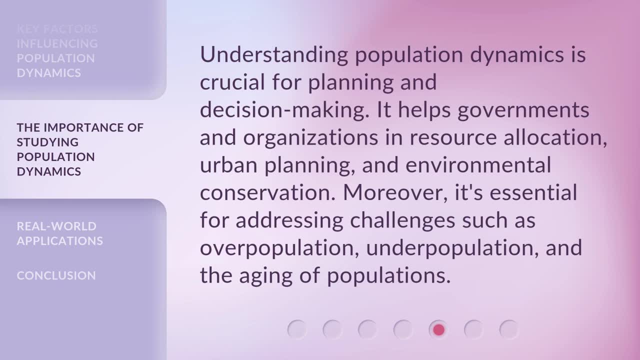 can have immediate and profound effects on population dynamics, influencing all the other factors mentioned. Understanding population dynamics is crucial for planning and decision-making. It helps governments and organizations in resource allocation, urban planning and environmental conservation. Moreover, it's essential for addressing challenges such as overpopulation, underpopulation and the aging of populations. 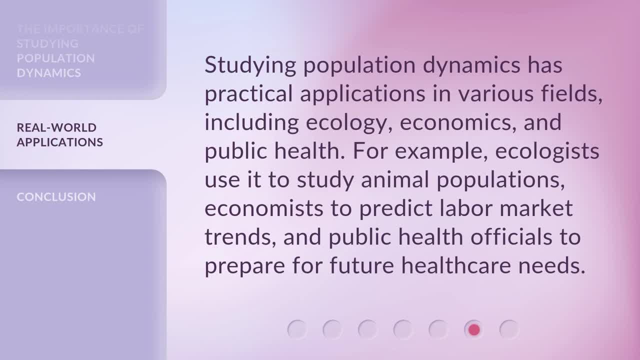 Studying population dynamics has practical applications in various fields, including ecology, economics and public health. For example, ecologists use it to study animal populations, economists to predict labor market trends and public health officials to prepare for future health care needs.